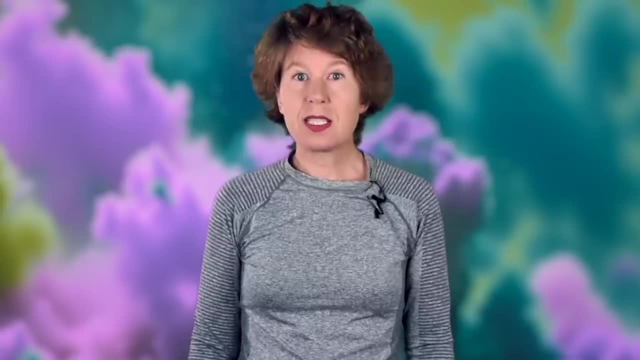 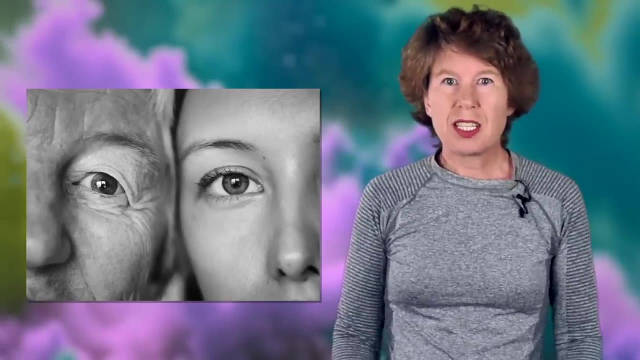 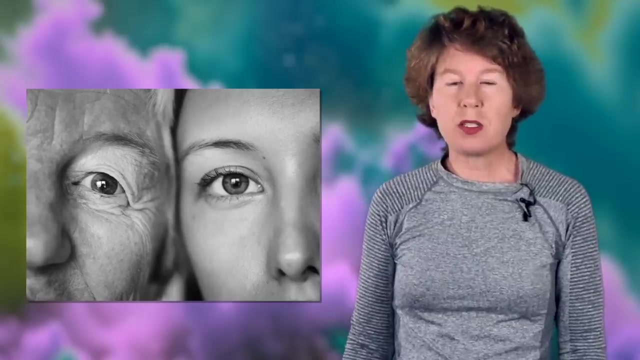 their own, but never repair themselves on their own. Physicists call it the arrow of time, and it's the reason why we get older but never younger. Its origin has remained somewhat of a mystery. According to the equations that we use to describe nature, it's totally possible, for 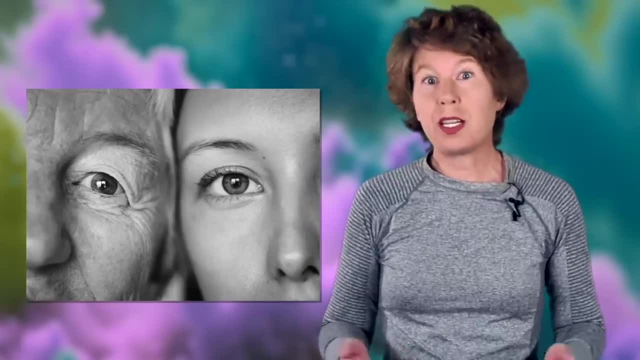 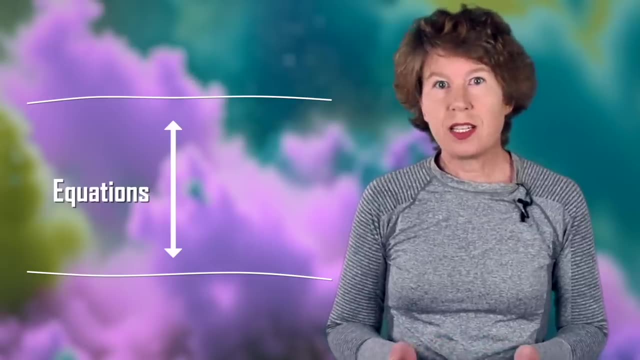 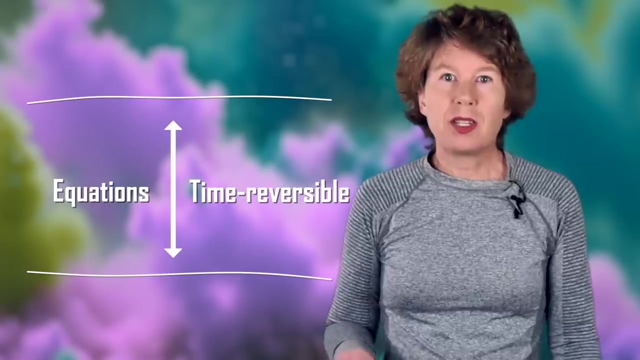 people to get younger, or for water drops to fly up into the sky. The equations we found work both forward and backward in time. We say that time reverses. We can totally write down an equation that makes water fly into the sky. In reality, though, this doesn't happen. So what gives? 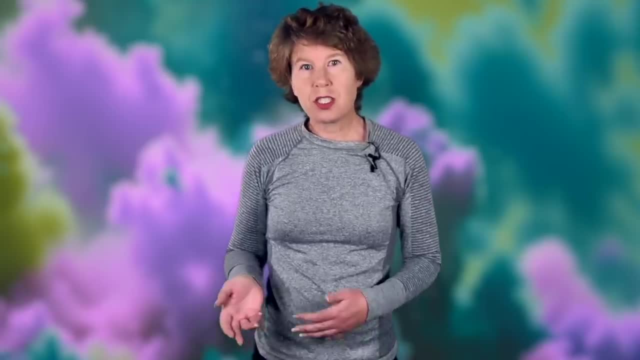 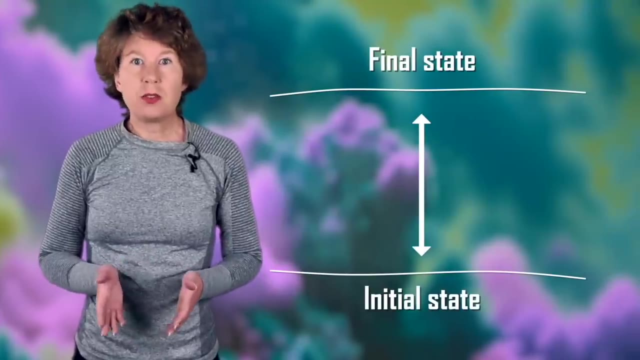 The reason is that to explain what goes on in nature, you don't just need an equation that tells you how things change. You also need what's called an initial state. You need to know what changes. This initial state is the entire configuration of the system at any one moment. 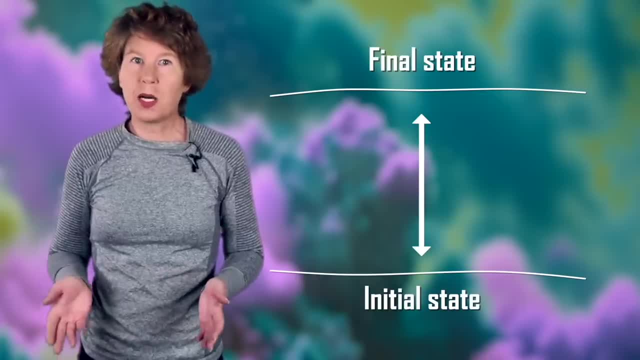 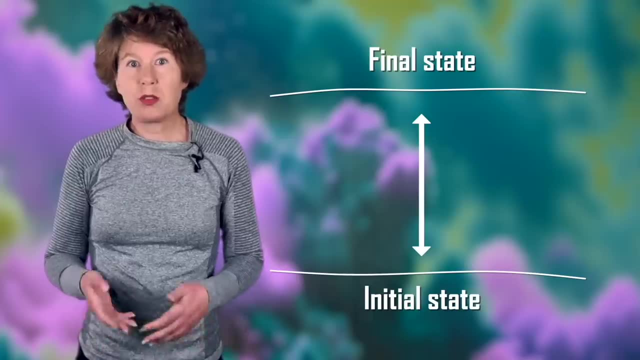 in time, For example the positions and momentum of all particles. You take this initial state and then you calculate what it does. Physics basically comes down to the unforgettable tick-tock. I had an initial state and guess what happened next? The thing is now that there are a lot of initial states that'll make water drop down from the sky, but very few that'll make it flow back up. To get this done, you'd have to very precisely arrange all the molecules in the ground to spit the water back out and the molecules in the air to 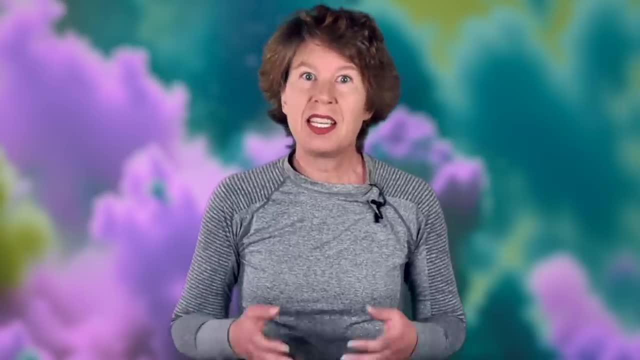 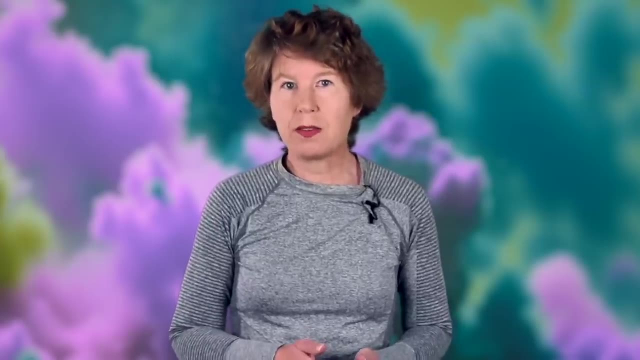 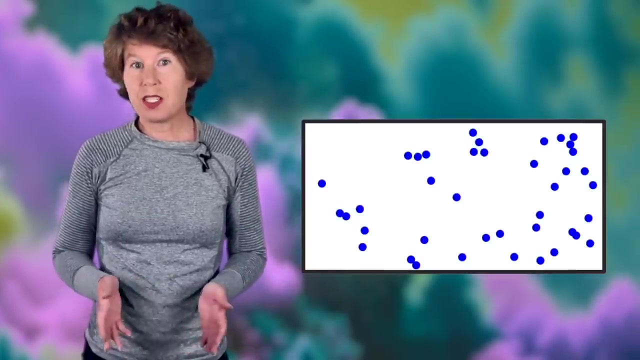 just the right drift for the drops to fly back up. It's so incredibly unlikely it never happens. Physicists quantify this probability with entropy. Entropy is a measure for how likely a system is to be in a certain configuration. Suppose you have a box and there's air inside. The air is made of molecules that move around. 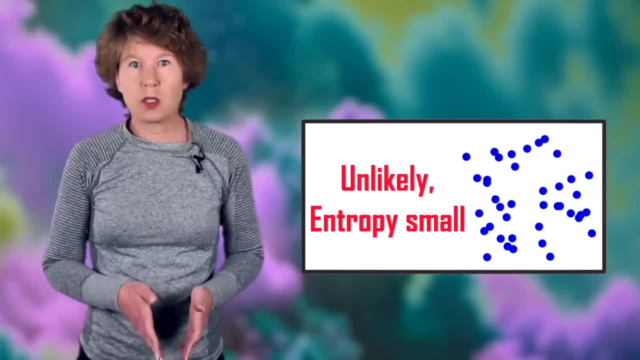 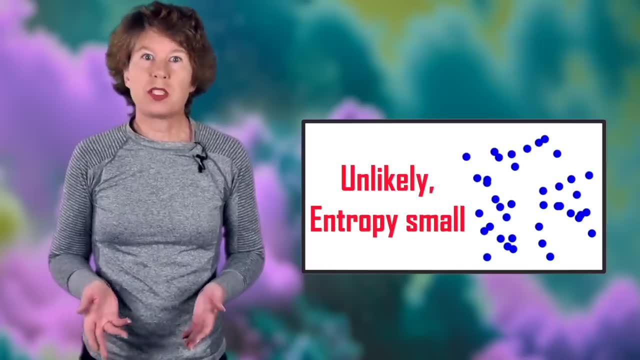 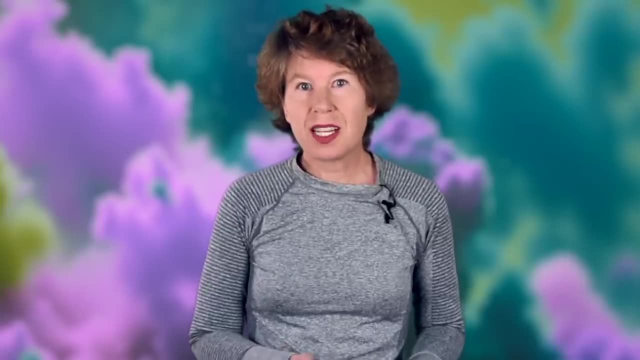 It's very unlikely that they all sit on the right side of the box. If that was so, the entropy would be small. It's very likely that they are almost evenly distributed in the box. The entropy in this case would be large. So what's going to happen if you put air in only one side of a box? Well, it's going. 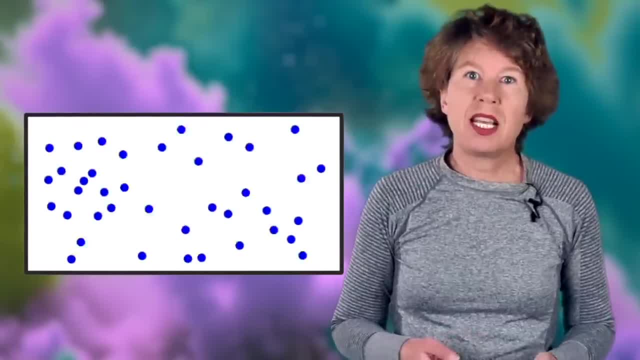 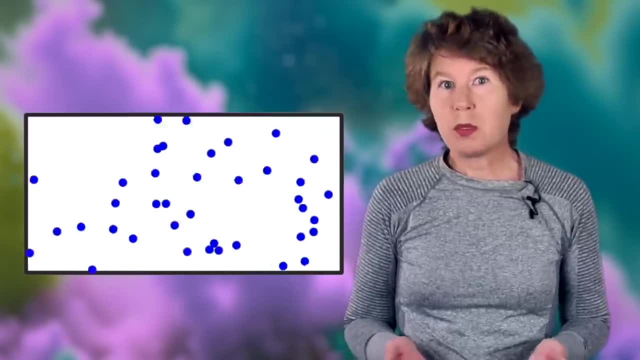 to spread out, because that's the likely thing to happen, And once the air is in a likely state, it's most likely to stay there. This means the distribution is going to remain approximately even, And luckily so, because it'd be inconvenient if you entered a room. 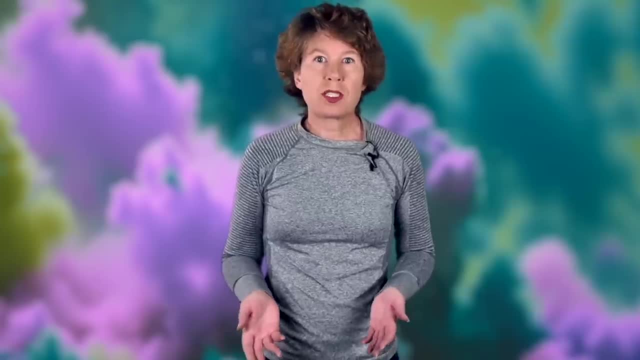 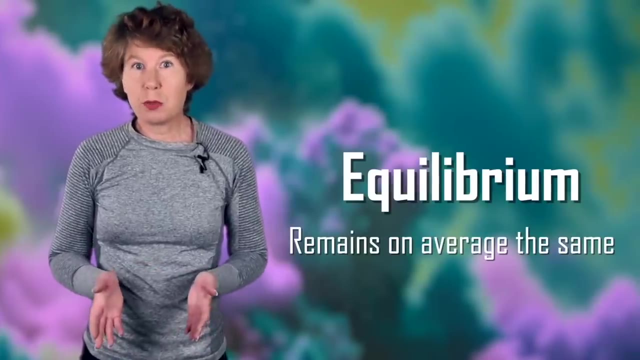 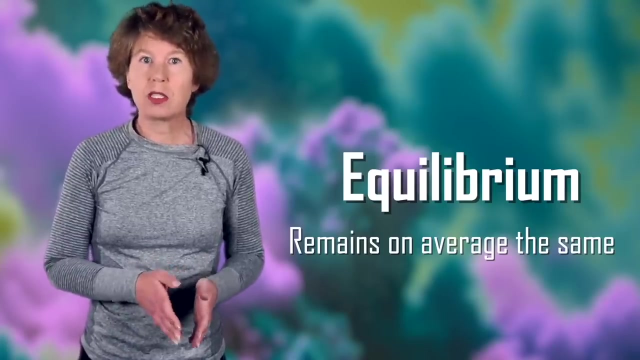 and all the air would spread out. The air went into a corner. We call such an approximately even distribution an equilibrium. It's not that the air molecules stopped moving when they're in equilibrium. they're still zipping around, but on the average the distribution stays the same for a very long time. 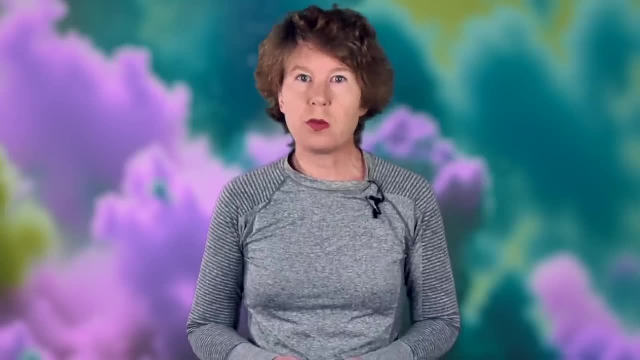 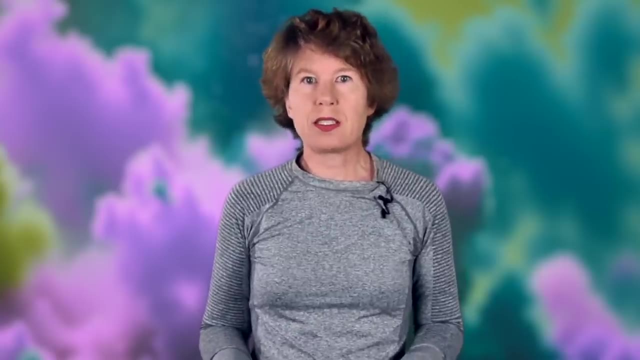 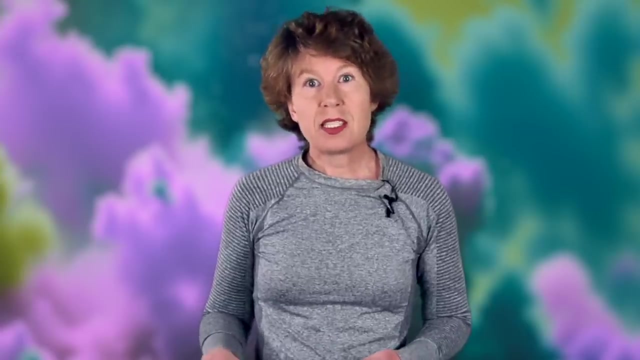 Physicists talk about entropy not just to confuse people on YouTube, but because it has practical purposes. If you have a system with small entropy, you can do work with it. In physics, work means useful energy. You can do something with it, For example, when the air is on one. 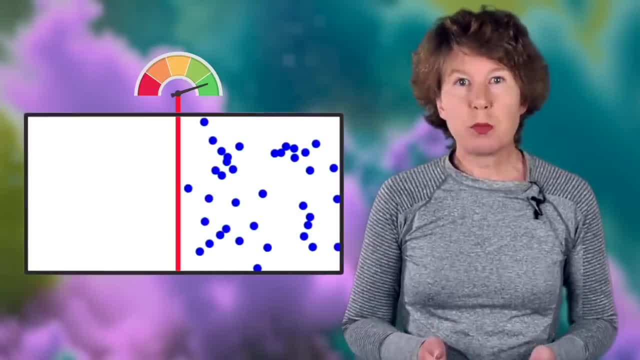 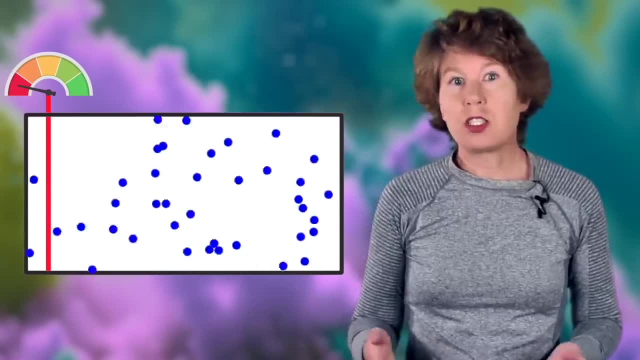 side of the box. you can put a divider in the middle and the air pressure will move it. You could convert this motion to electric energy and then do something else with it: Charge your phone, power a light, drill a hole into the wall and ruin your neighbor's. 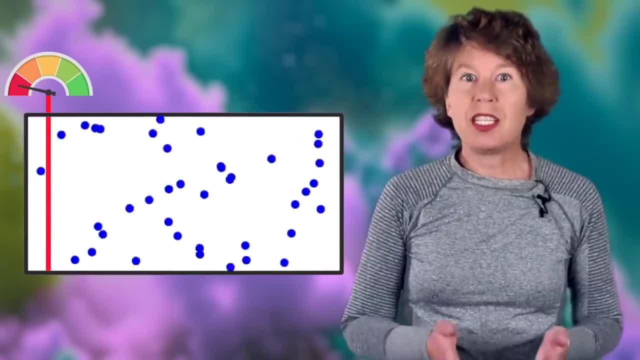 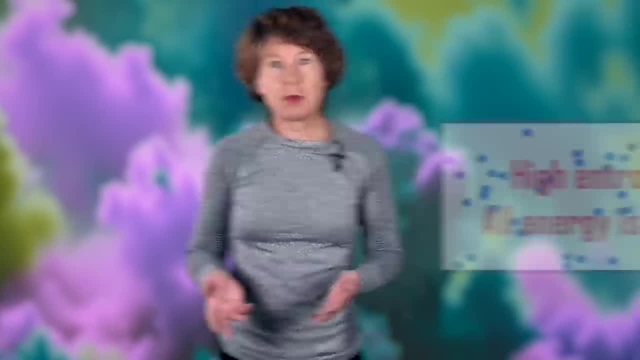 podcast recording. Every time you create structure, you do it by drawing on a reservoir of low entropy. So what's going to happen if the air is in one side of the box? Well, it's going to be the same. If the air has reached equilibrium and the average remains the same, there's 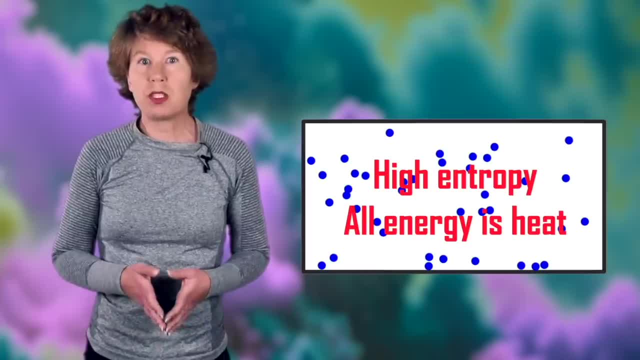 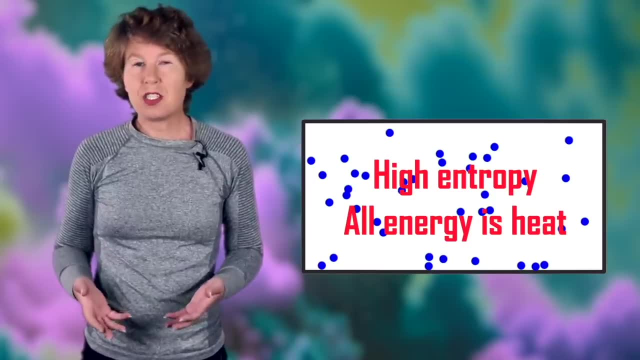 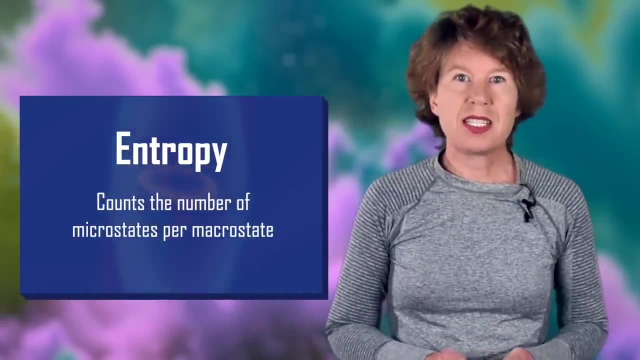 still energy in it because the molecules are still moving around. But it's not useful energy. You can't do work anymore. Physicists call this useless energy heat. Formally, entropy measures: the number of microstates per macrostate. A microstate is the exact. 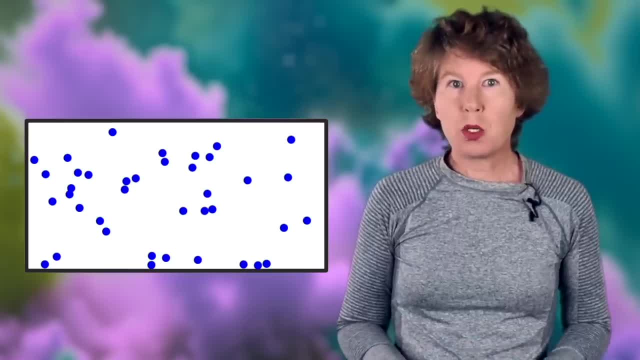 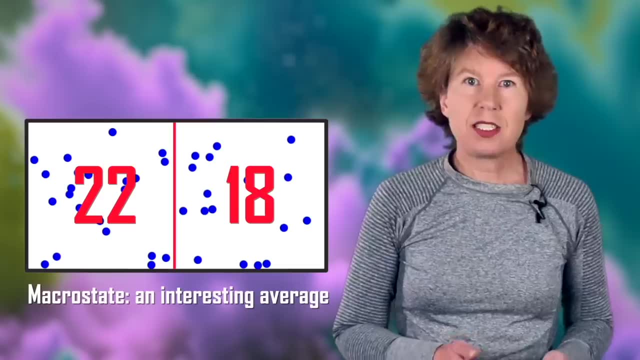 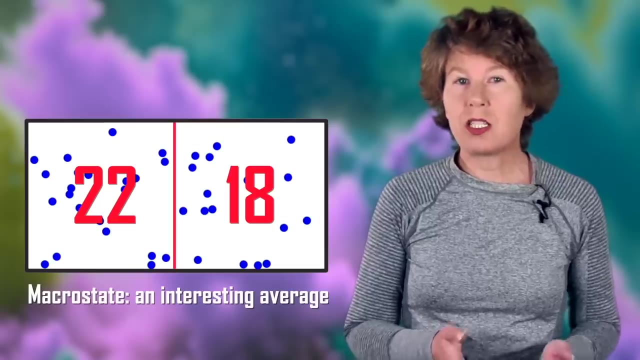 definition of the state of the system. For the molecules in the box, that could be the positions and momenta of each of the particles. A macrostate, on the other hand, is a state that we, as macroscopic objects, are interested in. For our box, that could be how many molecules are on the left and how many are on the right. 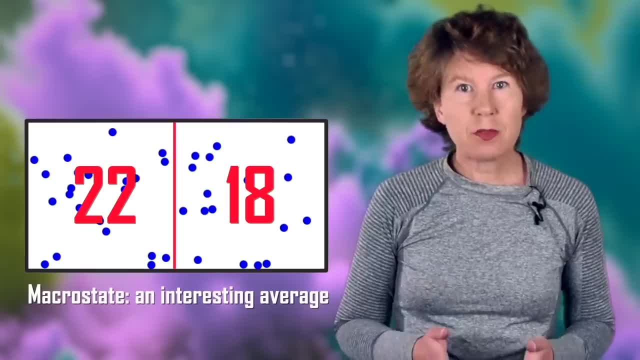 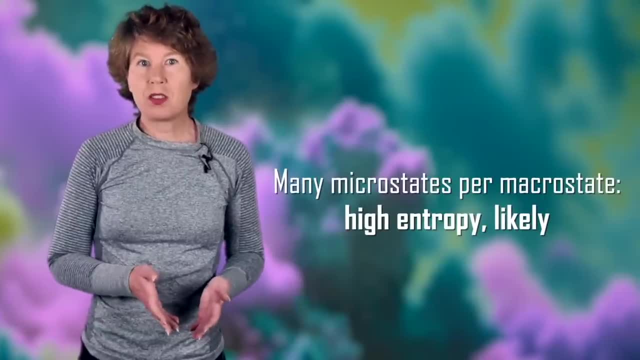 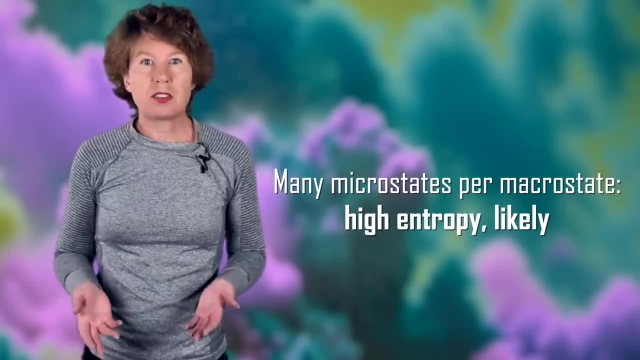 side of the box. A macrostate is an average over many microstates. If you want to know the entropy, you then ask how many possible ways there are for the air molecules to zip around so that there are approximately the same number on each side. 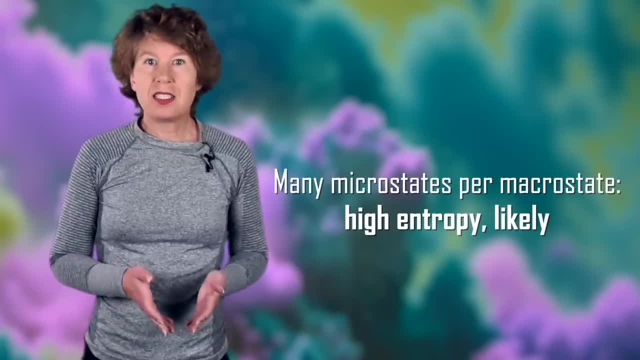 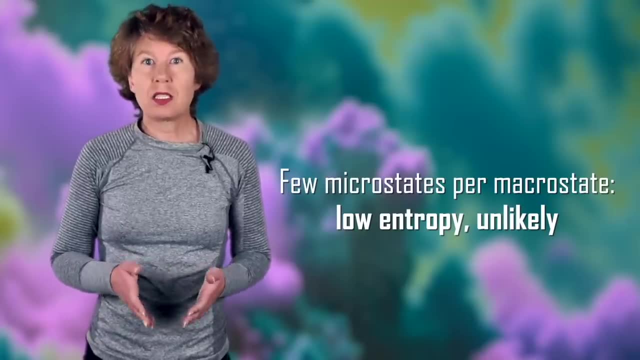 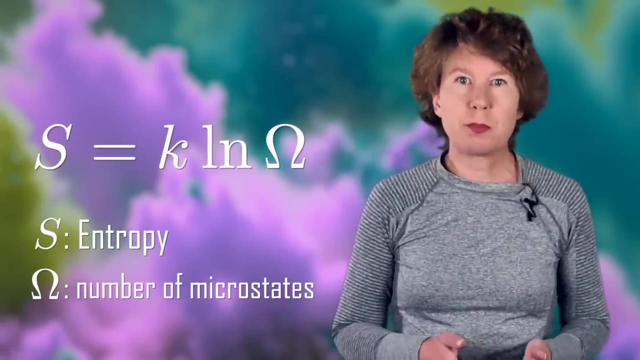 is there are a lot of those, so that's likely and the entropy is large. If they're all on one side, there are far fewer ways to get this done, so that's unlikely and the entropy is small. Technically, the entropy is the logarithm of the number of microstates multiplied by 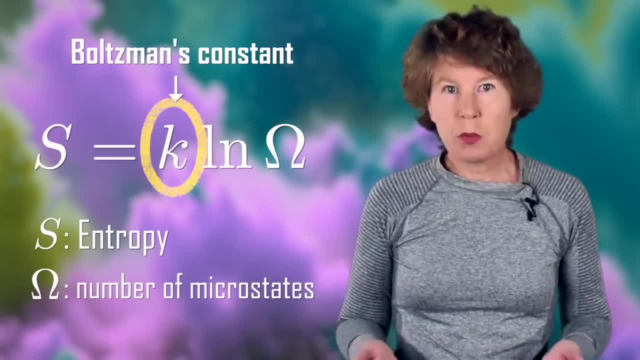 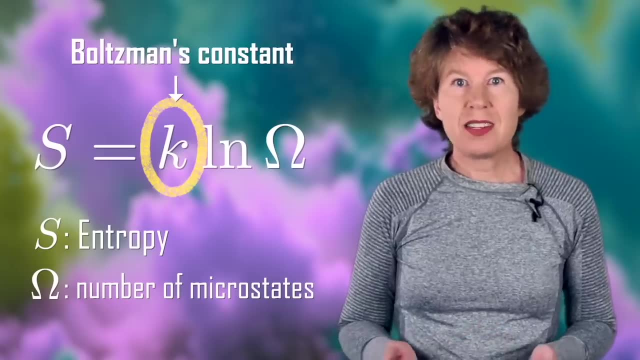 a constant called Boltzmann's constant. If you remember one thing about the logarithm, it's probably that the logarithm of one is zero. This means the entropy is zero if, and only if, there is exactly one microstate for your macrostate. 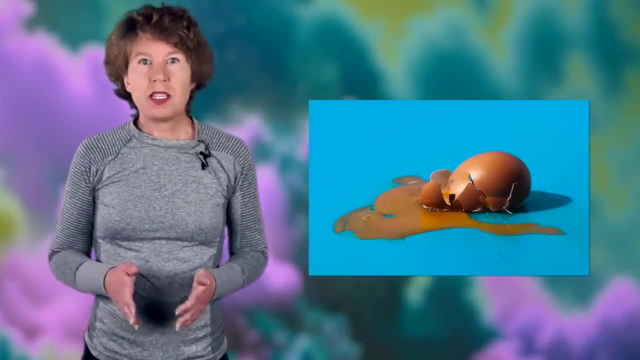 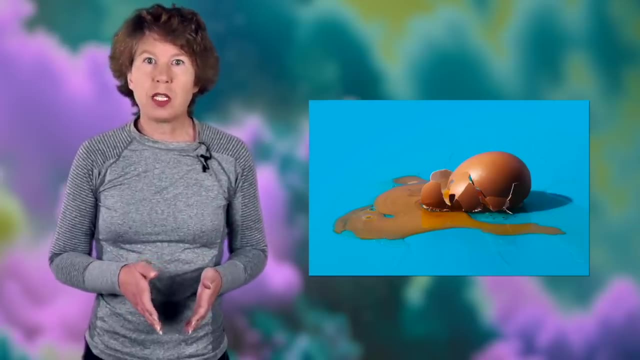 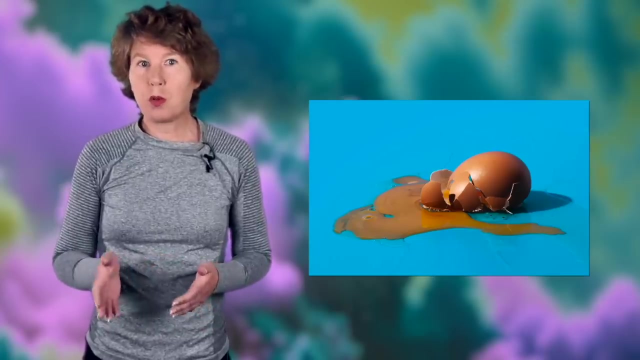 Okay, so why does entropy increase? Entropy increases because that's the likely thing to happen And that removes part of the mystery about the error of time, because it explains why we observe some things and not others, even though the laws of nature work both forwards. 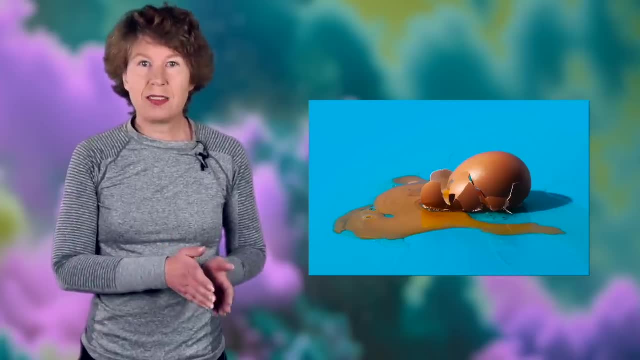 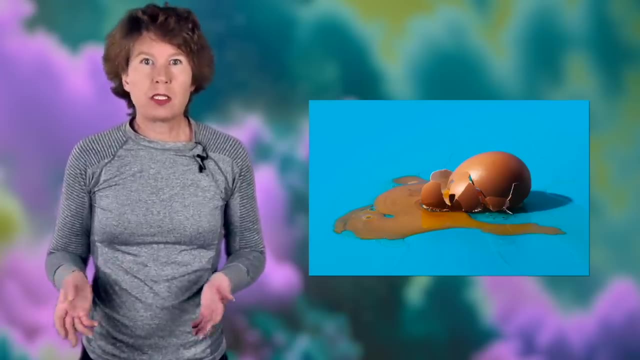 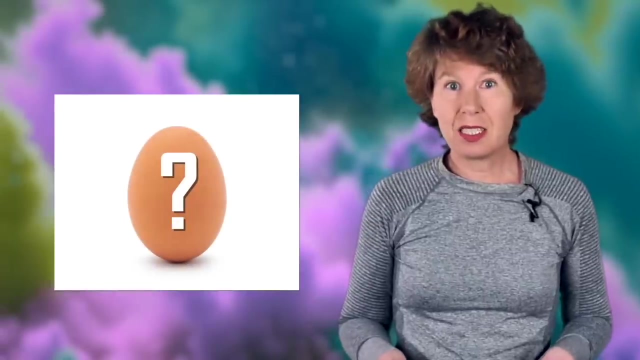 and backwards in time time, Because one way is more likely than the other. An egg that falls to the ground breaks. It doesn't jump up and unbreaks. Alright, we sorted it out. But this brings up another question. If low entropy states, like eggs, are unlikely, why? 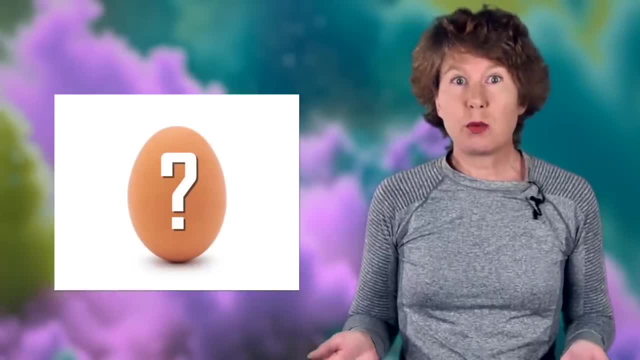 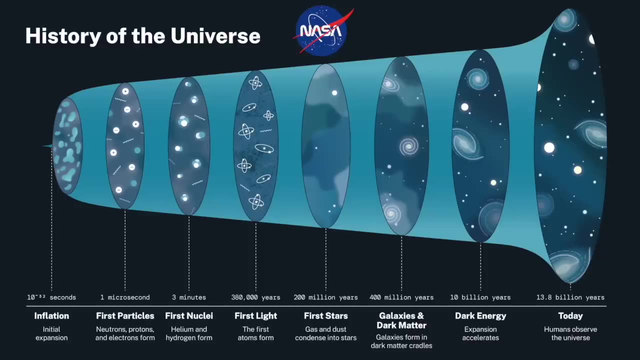 do we have them to begin with? Why isn't the universe in equilibrium already, when that's most likely? We don't know. We do know that the universe must have started in a state of low entropy, a very unlikely state, but we have no idea. 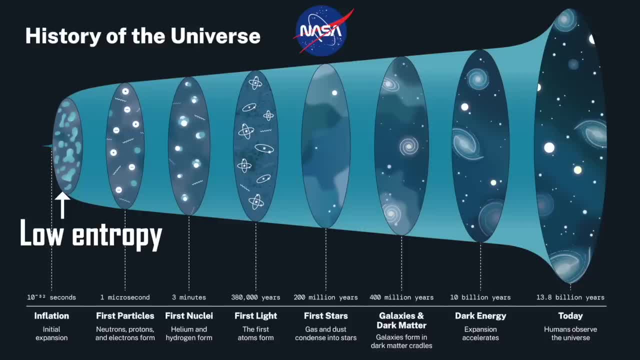 why It's often called the past hypothesis, a term introduced by the philosopher David Allbirds. It just posits that this is what it was, but it doesn't explain why The entropy of our universe has been increasing ever since the big bang, because that's what's. 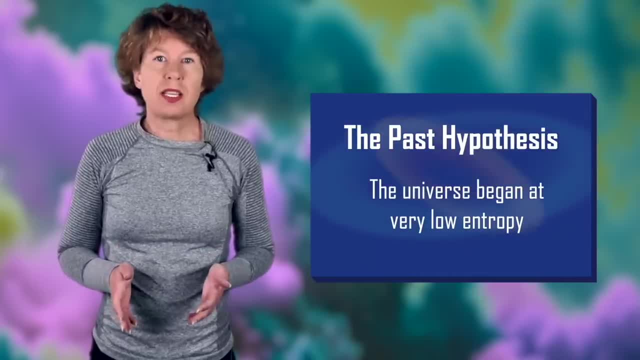 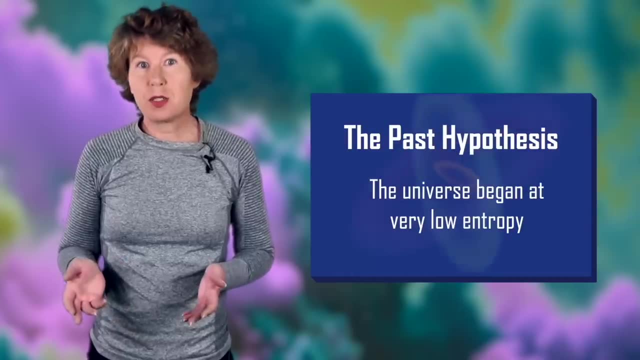 likely to happen, But this is the total entropy. In some parts of the universe, entropy can and does remain small for a very long time. So the entropy of our universe should be lower than the entropy of the universe So long time, because it doesn't have to be evenly distributed. Indeed, we can shovel around entropy. 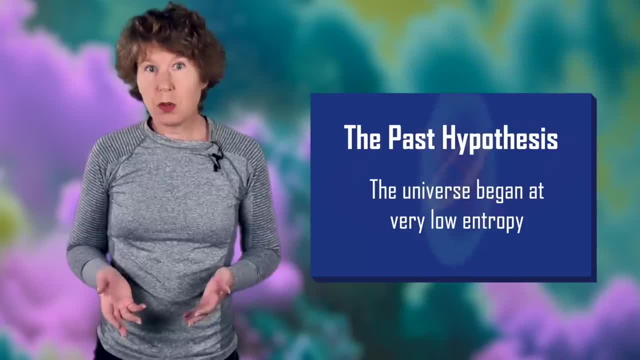 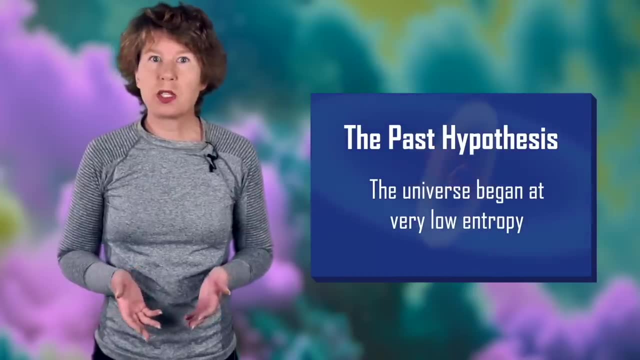 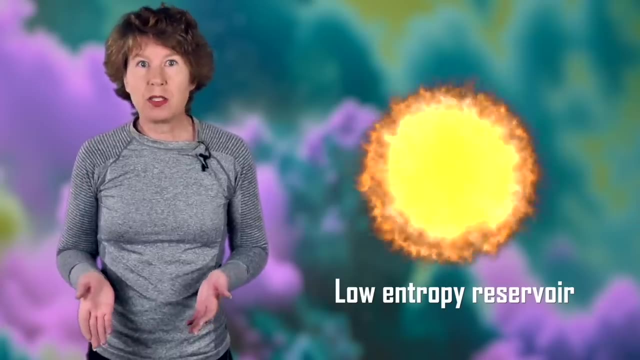 ourselves. If you have a reservoir of low entropy, you can use that to lower the entropy elsewhere, And luckily we have a big low entropy reservoir nearby, though it's more commonly called the Sun. The Sun started out at low entropy. As it fuses atomic nuclei, its entropy increases. 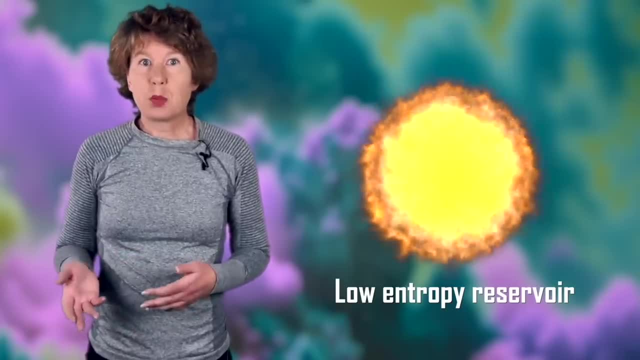 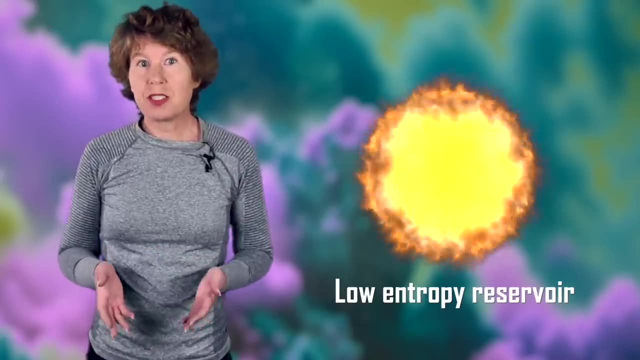 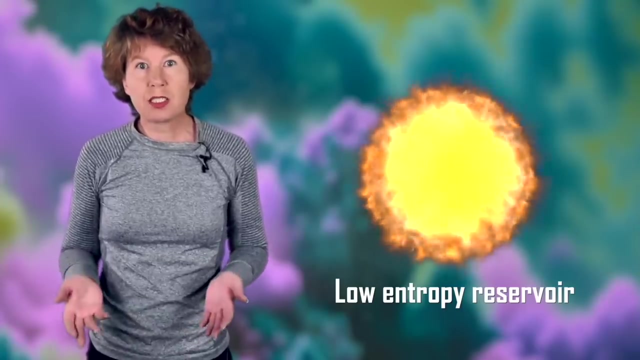 Again, that's because that's the likely thing to happen. As the entropy of the Sun increases, it sends energy with low entropy to us in form of sunlight. We can use that to create electricity and lower the entropy of something else. We can use it to run a fridge and keep the eggs cool. 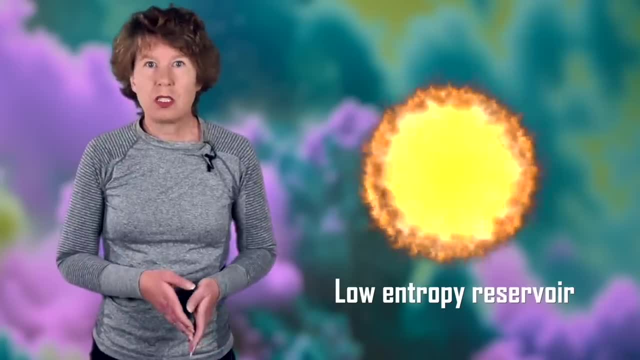 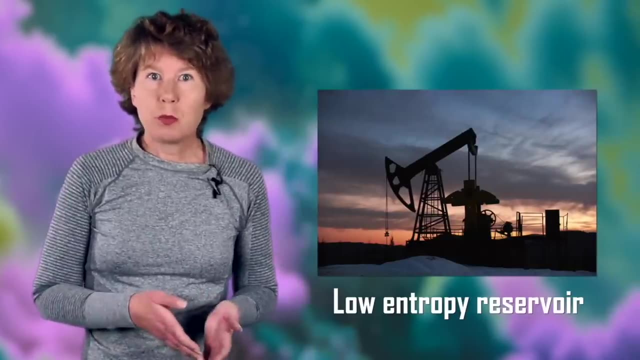 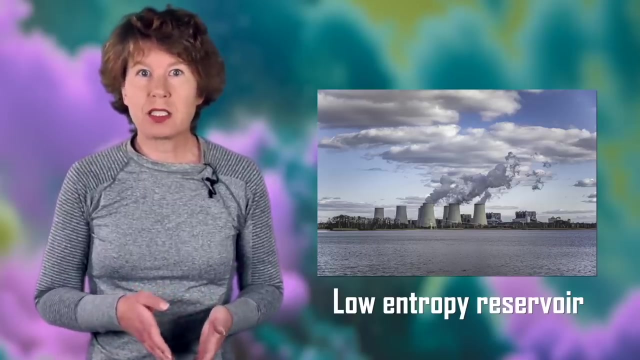 or power a light and find out what's under the couch, Or maybe better not. It's a similar story with fossil fuels. They're low in entropy. If we burn them, we increase the entropy. Of course, the sun has the entropy of those fuels or their remains, and we can use that to decrease. 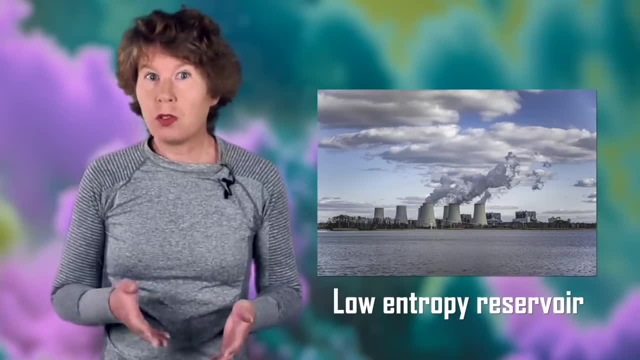 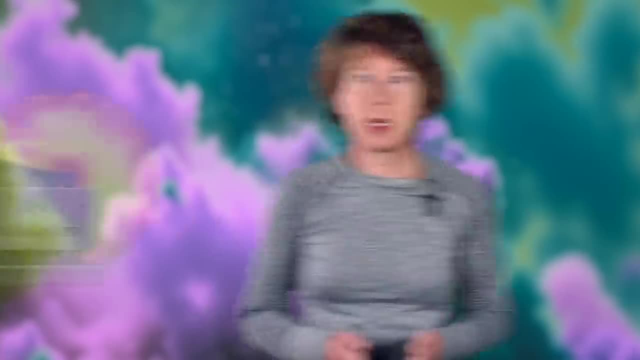 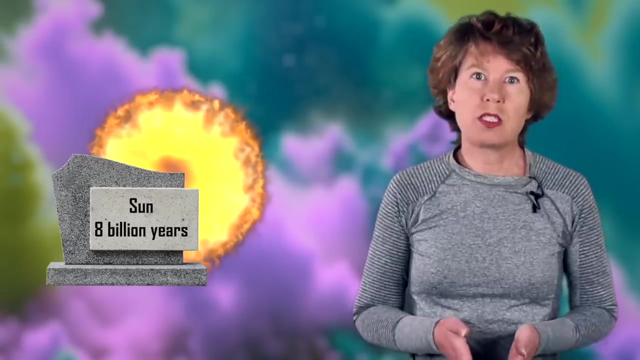 the entropy of something else. For example, we can manufacture goods or products. These are all low entropy objects with specific structures that we have created. But eventually this'll stop working because we'll run out of low entropy reservoirs. Our sun will run out of fuel. Earth's 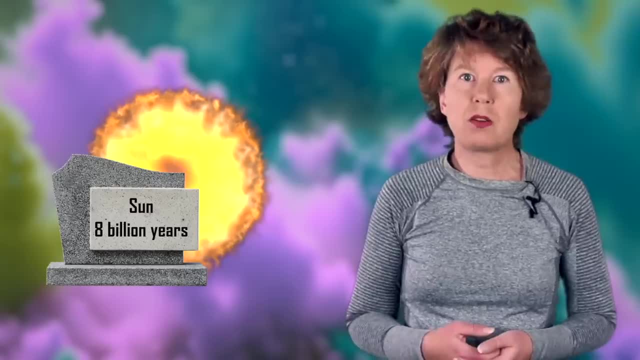 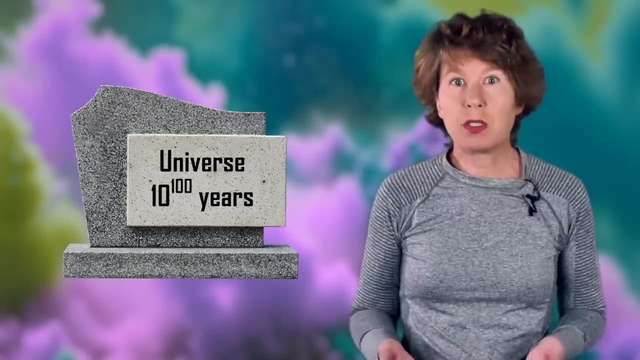 core will go cold, Other stars will run out of fuel too, And eventually 10 to the 100 years or so from universe will come into thermal equilibrium. entropy will be as large as it can get and nothing will happen. on the average, 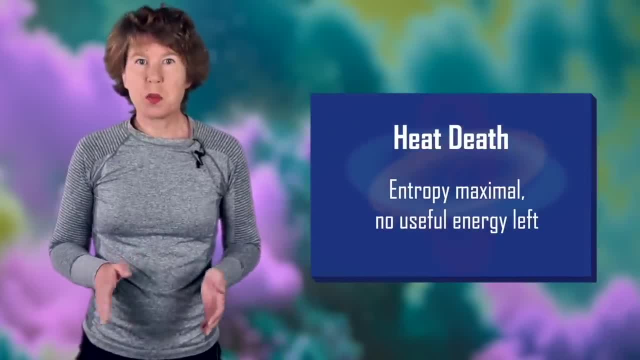 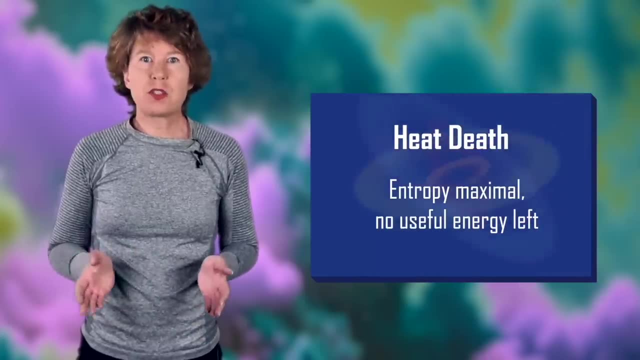 Physicists call this heat death. The word is somewhat misleading because it doesn't mean it'll be hot. to the contrary, it'll be very cold and very dark. Heat refers to the useless energy that I mentioned previously. It'd better be called high entropy death. 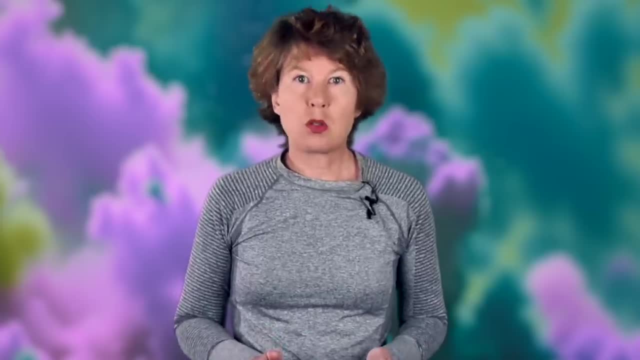 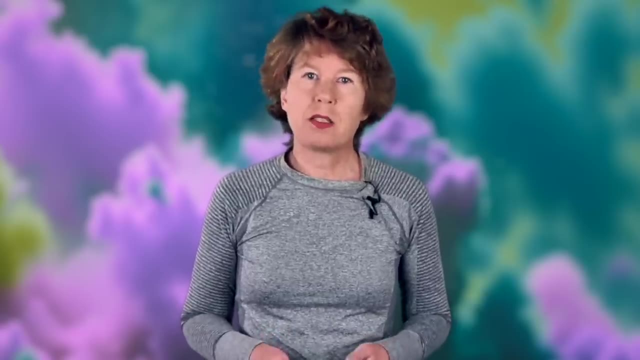 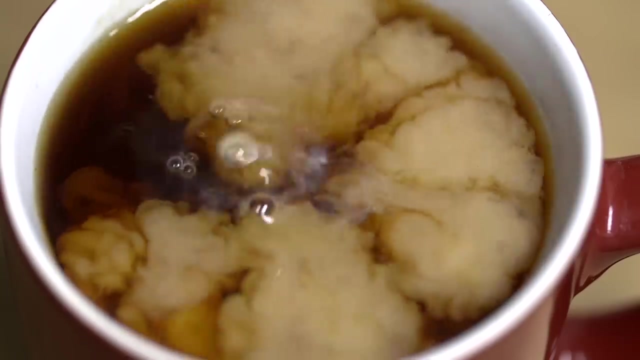 What does entropy have to do with order? This has always confused me. I now think the brief answer is nothing, Because order doesn't have a well-defined meaning. For example, imagine you're pouring milk into tea. At the beginning they are neatly separated, ordered, you could say. 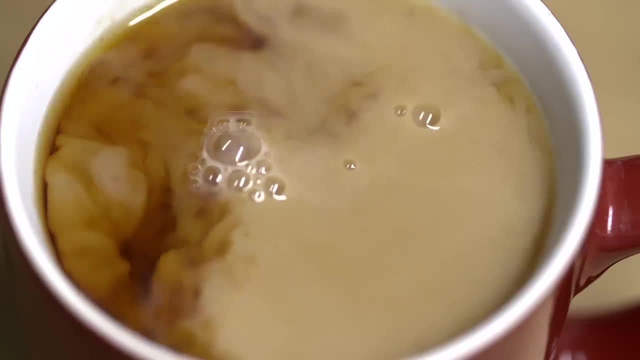 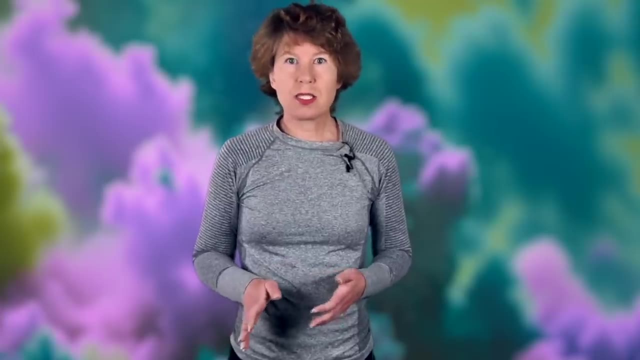 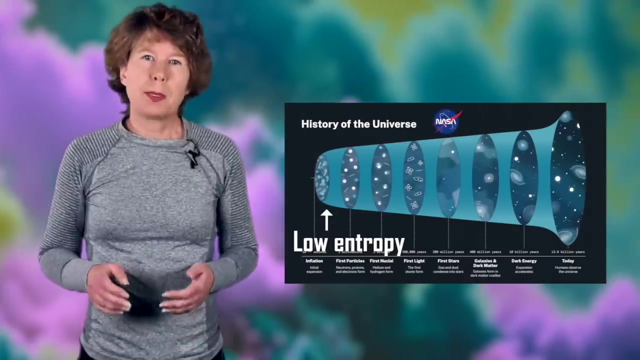 At the end they are evenly mixed. I'd also call this ordered, But in physics this even distribution doesn't count as order. This reference to order causes a lot of confusion. For example, as we saw earlier, The entropy in the early universe must have been small. 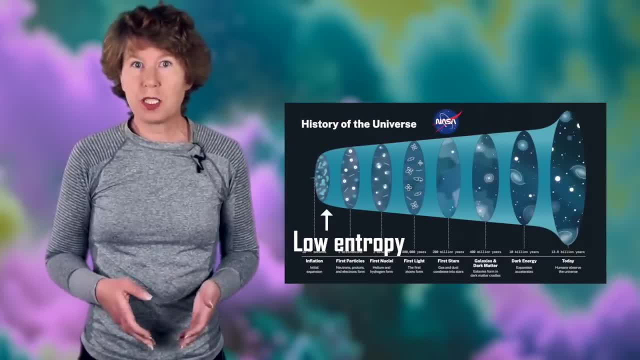 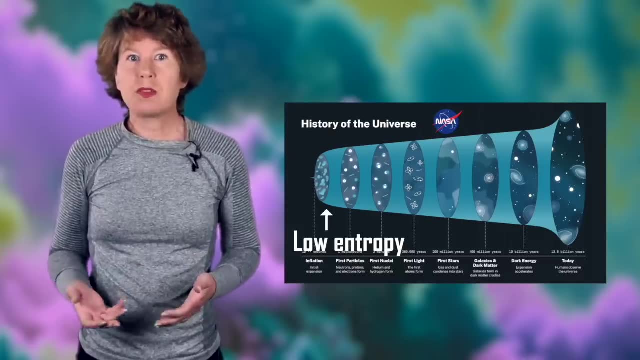 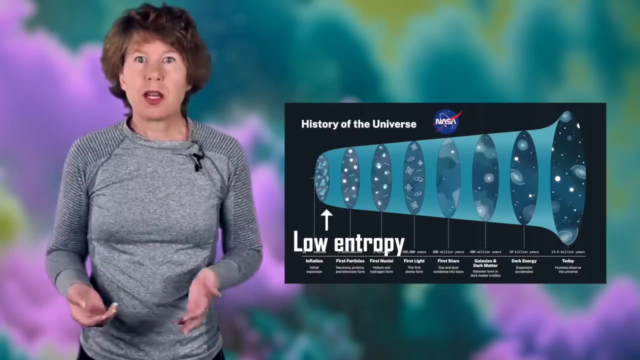 Back then, matter was very evenly distributed, with small fluctuations in the density which then grew to galaxies. At the end of the universe, matter will again be evenly distributed, with small fluctuations in density. Both cases seem equally ordered, if you wish. So how can it be that one has low entropy and the other high? 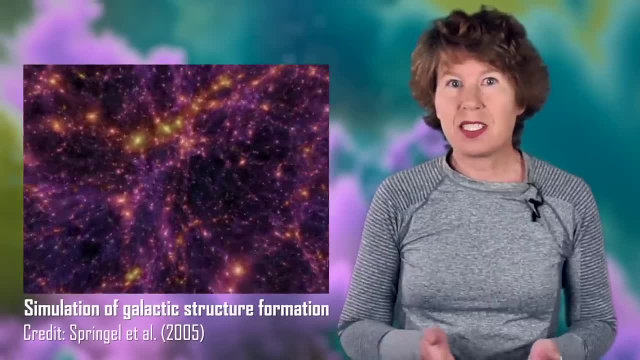 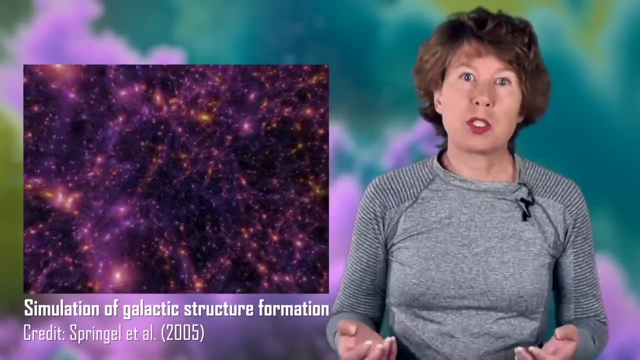 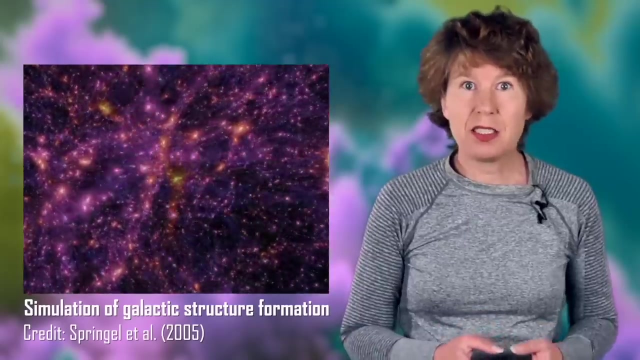 It's because in the early universe the density of matter is high and this means the gravitational force is strong And the gravitational force is attractive, so it wants to draw the stuff together. An even distribution of matter when gravity is strong is incredibly unlikely. 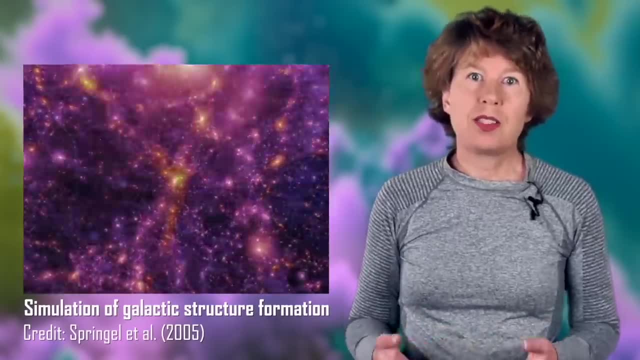 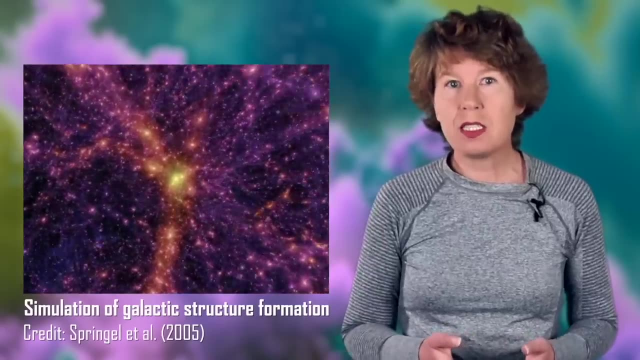 It's unstable. It wants to clump. This even distribution therefore had low entropy. At the end of the universe, however, matter will be very thinly distributed and gravity will be weak, so it doesn't want to clump again. 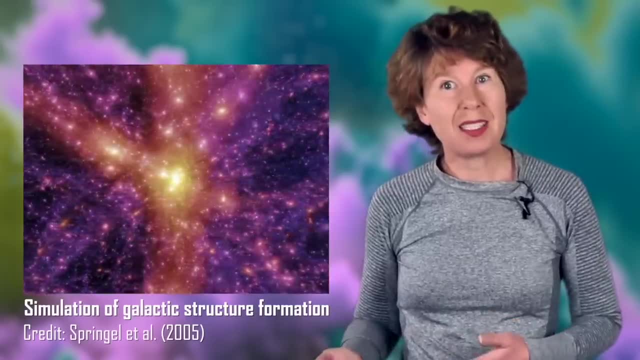 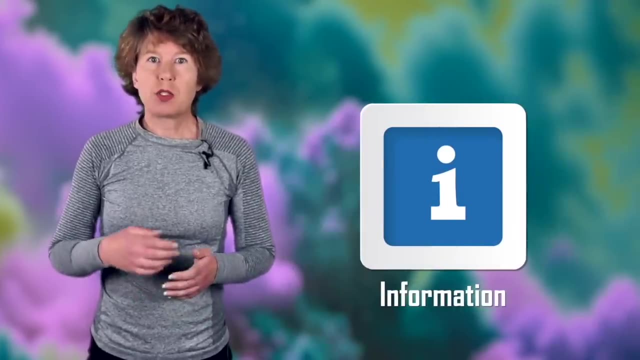 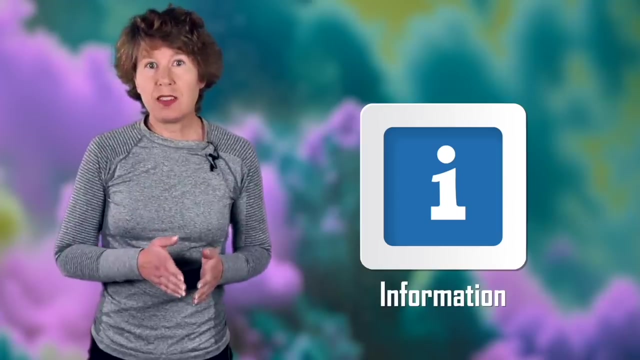 This is a very likely situation. So the entropy is high. And what's with information? Ah yes, the relation between entropy and information is subtle. It comes from the definition of entropy as the number of microstates per macrostate. Remember that to calculate the entropy, you average over microstates. 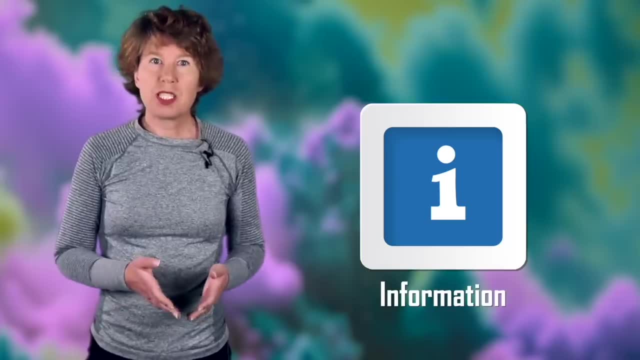 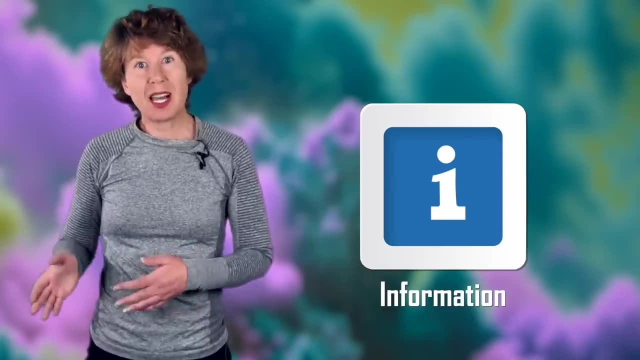 This means you throw away information. In a macrostate there's something you don't know, So high entropy means low information, And low entropy means low information, And low entropy means high information. All that I told you so far is pretty standard textbook stuff. 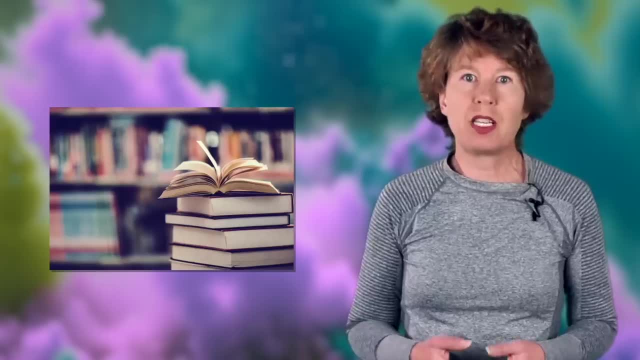 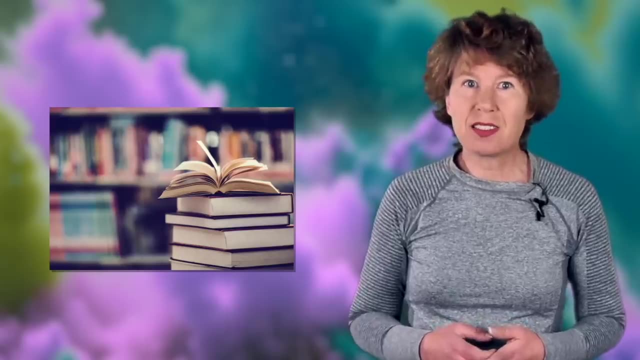 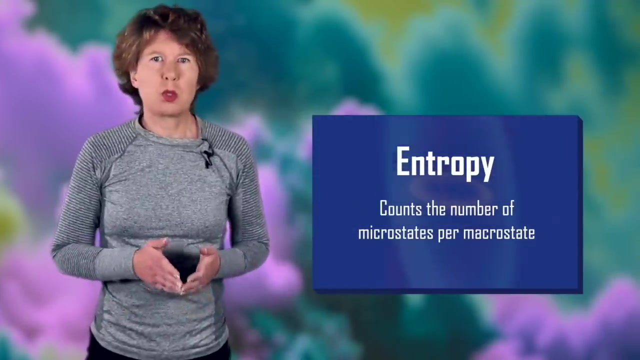 And if you pick the random physicists on the street and ask them if they agree, you should let them go because they have better things to do. Now I want to tell you why I don't think heat death is how life will end. Remember that entropy counts the number of microstates per macrostate. 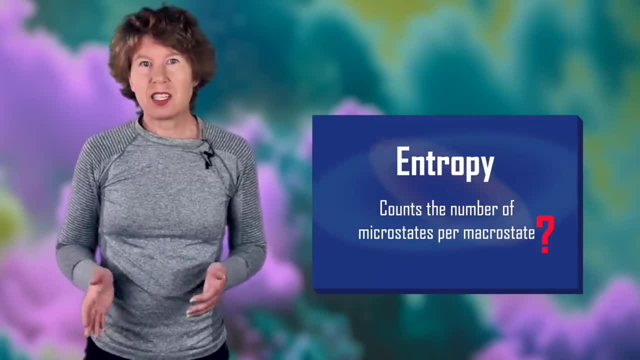 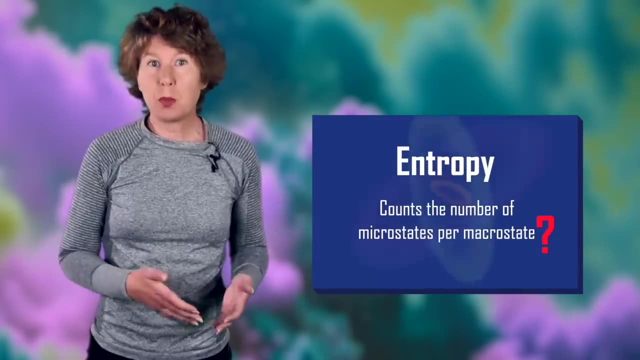 But what is a macrostate? A macrostate is a state that we, as humans, are interested in. It's something we call a macrostate. It's something we choose to calculate, a quantity that's useful for our purposes. It's an average description that we're interested in, maybe because we want to understand. 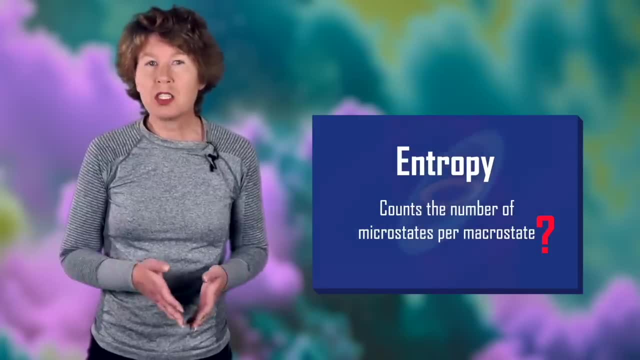 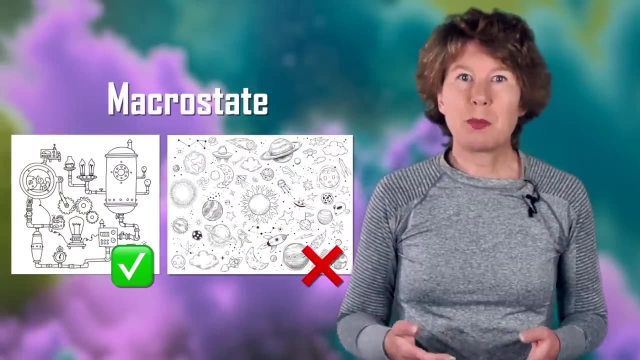 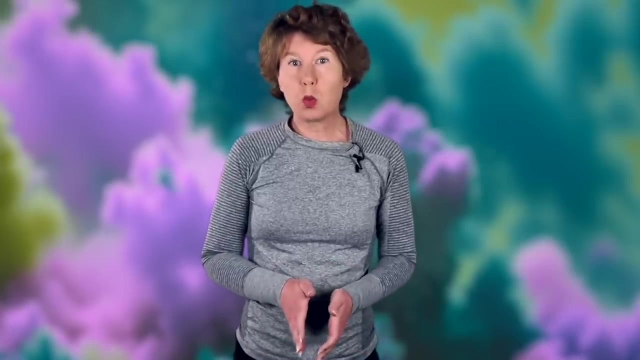 how efficiently a fridge will work or how much power an engine will have. Those are good reasons, but a macrostate has no fundamental significance and it makes no sense to use it to talk about the fate of the universe. See, a system is always only in one microstate. 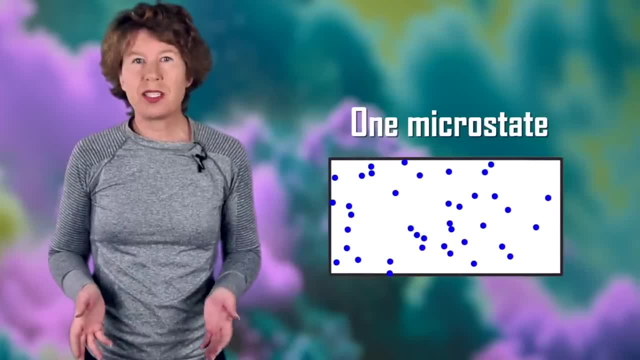 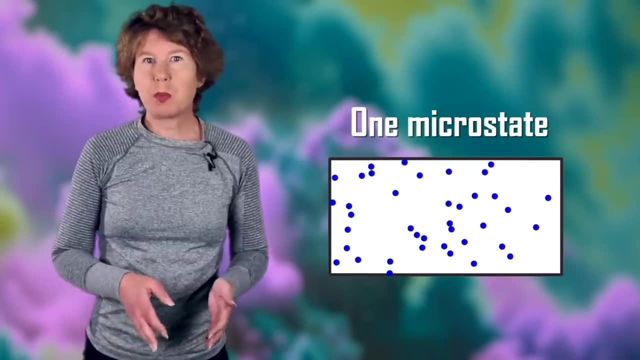 That's true for the molecule of a macrostate, That's true for the molecule of a macrostate, That's true for the molecules in the box and also for the entire universe. They're in one particular configuration, one particular state. The probability of this microstate is one and that of all other states zero. 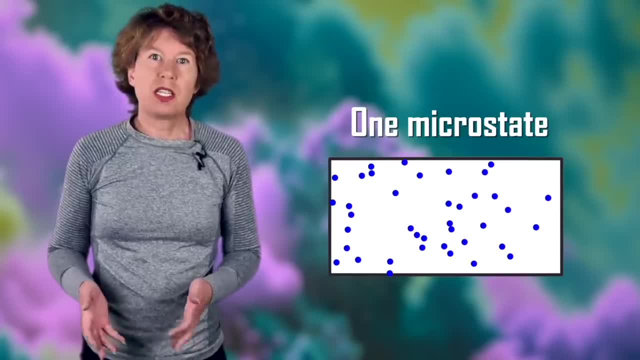 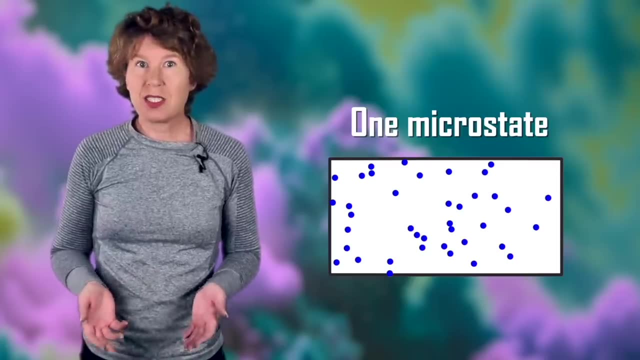 And as the state changes in time, this will remain so. The entropy of this one microstate per microstate is always zero and stays zero. The second law of thermodynamics doesn't say that entropy increases, It says it doesn't decrease. 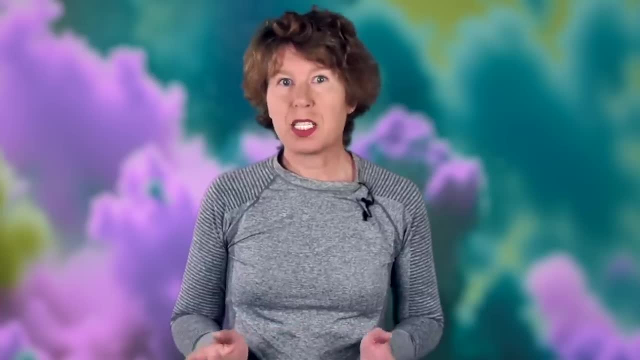 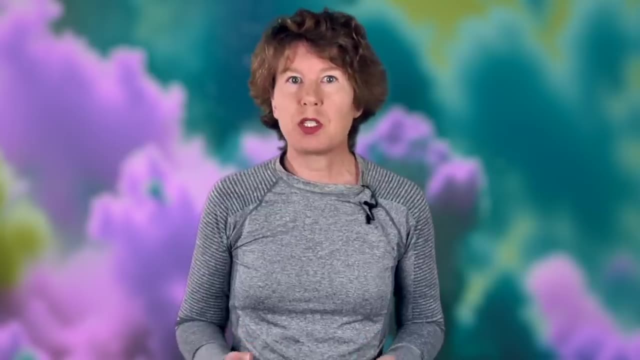 But it can full well remain zero. The reason we get more complicated probabilities and the reason we say entropy increases is because we lack information about some systems. If we put air molecules in the corner of the box, we don't know where they're going. 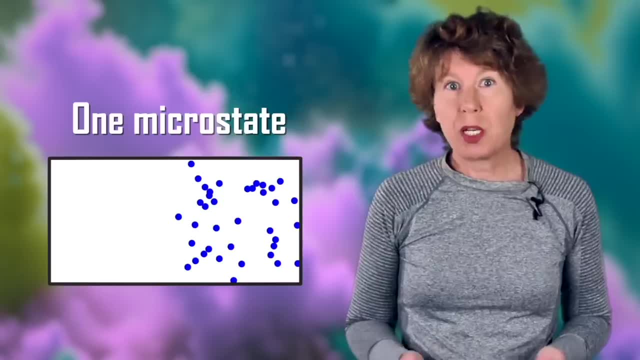 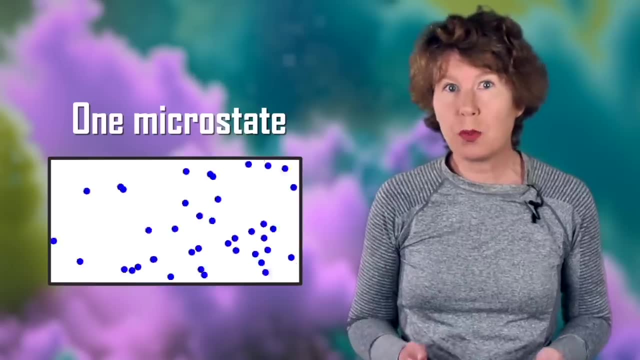 but at least we know where they are. If we now let the air spread into the entire box, it's still the same microstate. It's still a microstate that one minute ago was in the corner of the box. but we can't. 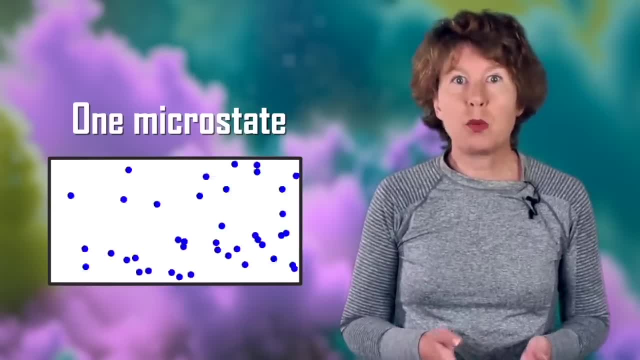 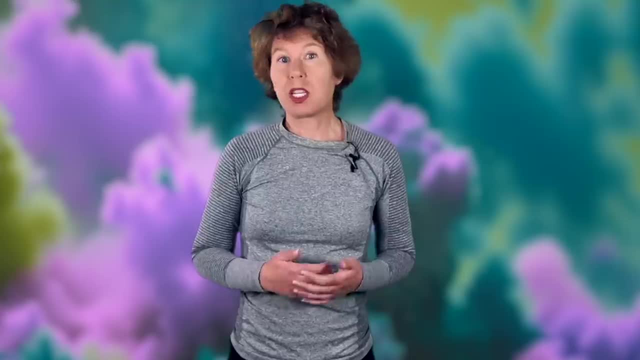 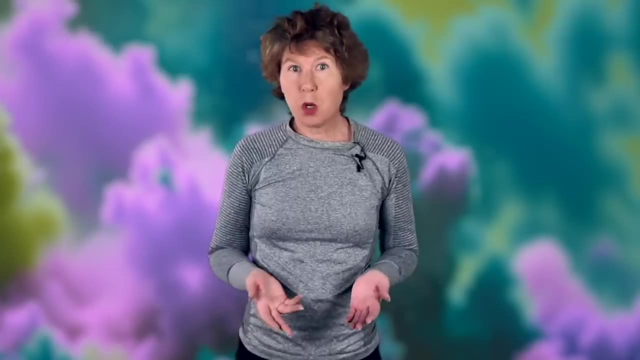 tell. We used to have information about this state. we no longer have. That's why entropy increases, because we lose access to information. But there are always microstates that'll turn a high entropy system into a low entropy system For the molecules in the box. for example, you could put in a divider like this: 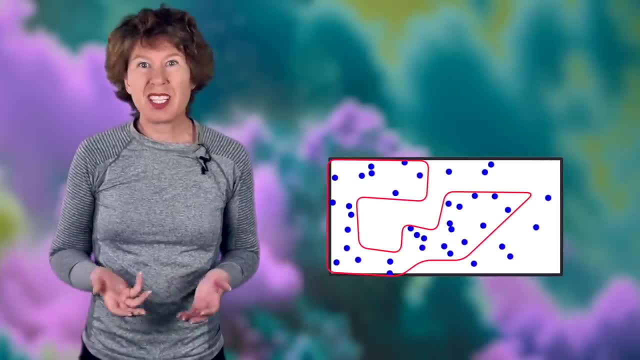 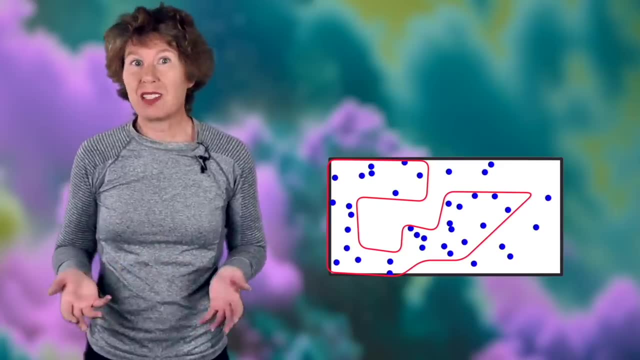 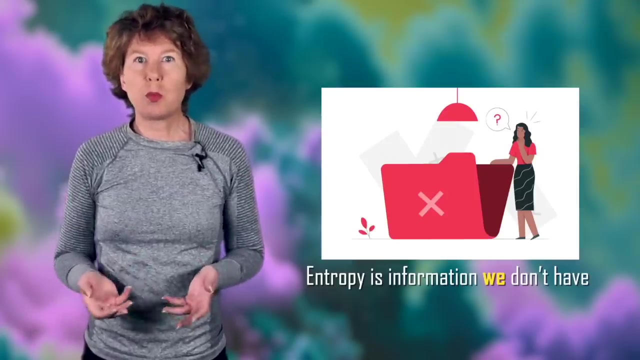 It's just that this would require information that we cannot easily access. We can access it, but for that we'd need another low entropy reservoir, So nothing would be gained. The relevant point is now that our notion of entropy is based on the physical properties. 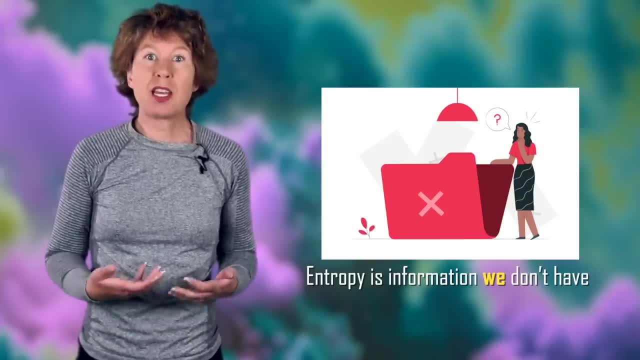 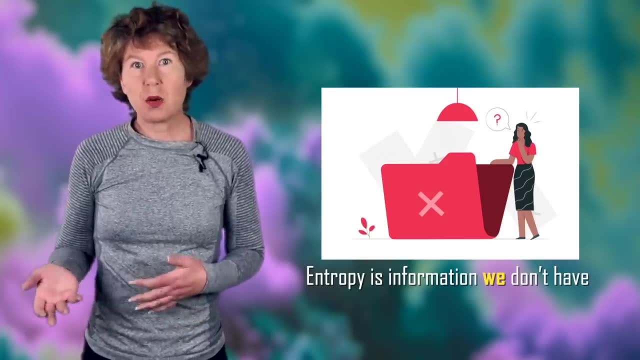 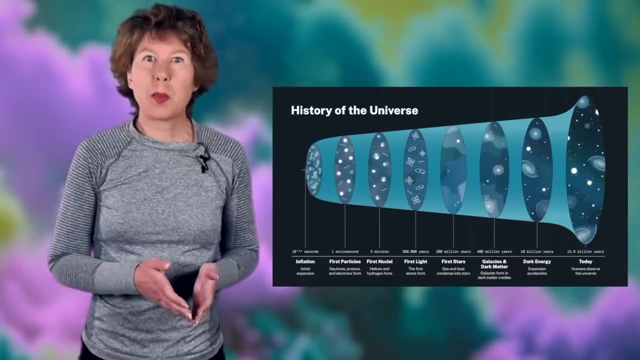 of macroscopic devices that we humans have easy access to. It isn't a fundamental property of nature. I believe that as the universe gets older and entropy increases according to us, new complex systems will emerge that rely on different macrostates, macrostates that we ourselves 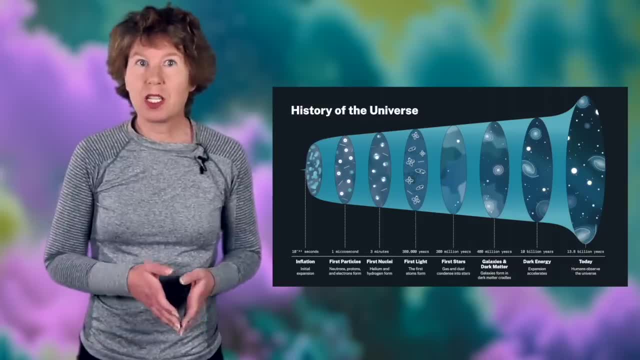 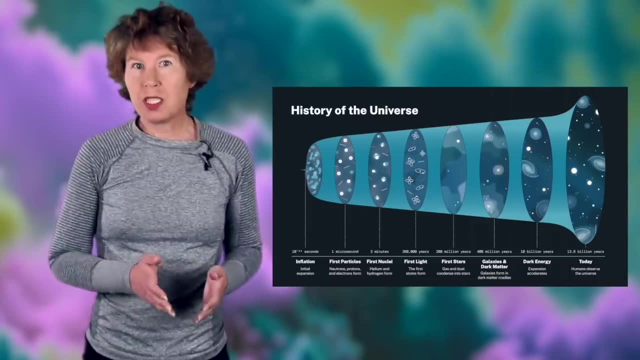 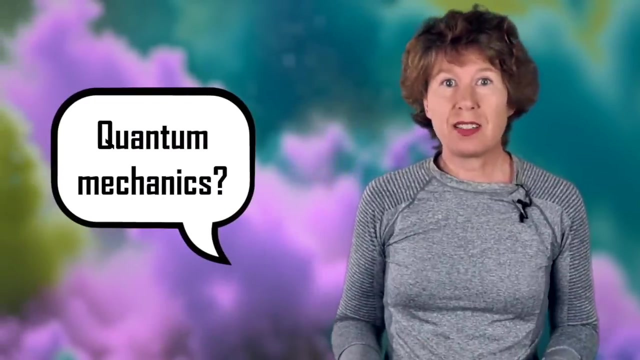 could never use. And for those complex systems- call them living beings- the entropy will be small again. So life will go on, but in a form very different from us. And what about quantum mechanics, I hear you ask. Quantum mechanics doesn't change anything about this. 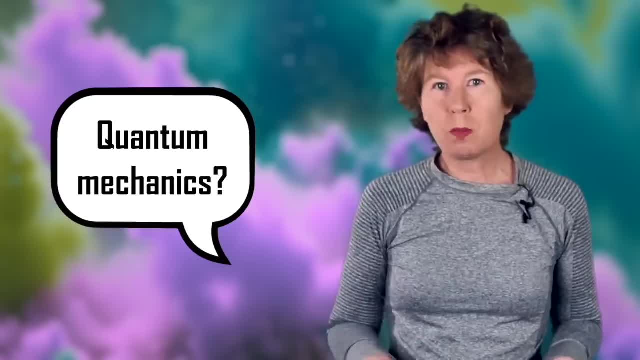 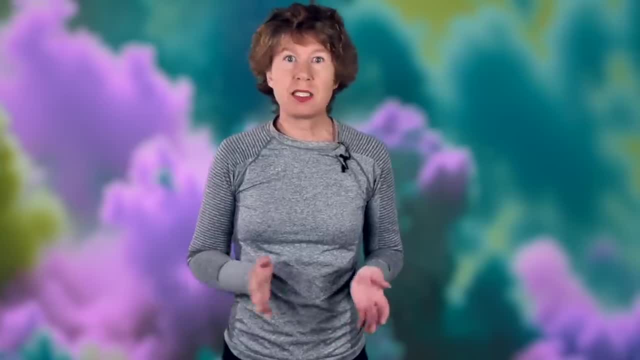 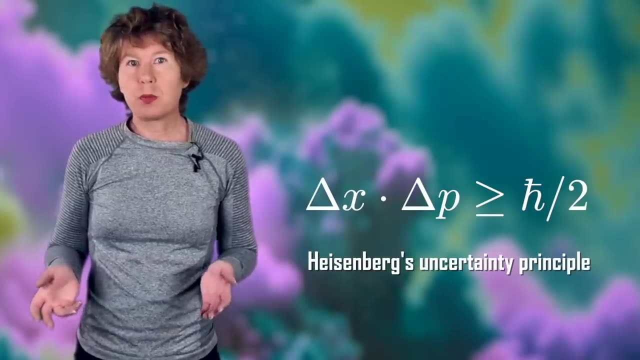 In quantum mechanics the universe is still in exactly one microstate, It's just that now it's one big wave function. I sometimes hear people say that the Heisenberg uncertainty principle implies that the universe can't measure quantities at the same time, for example position and momentum. 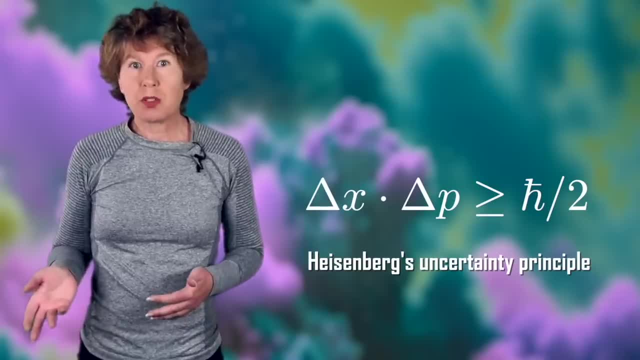 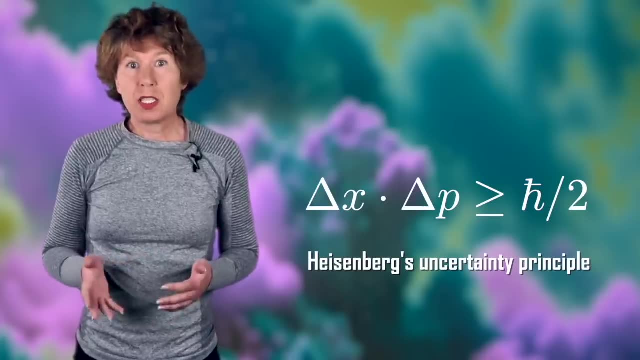 But this is a misunderstanding. You can totally measure both. it's just that if you can predict the outcome of one of those measurements very well, you can say very little about the outcome of the other measurement. I talked about this in more detail in an earlier video. 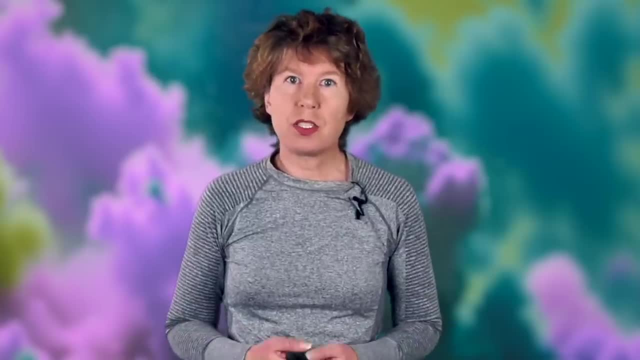 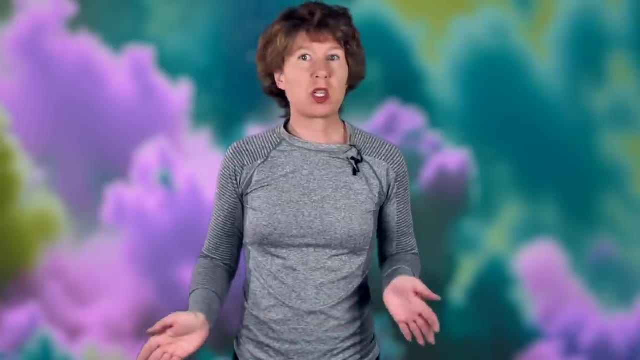 So if in ten to the one hundred years you arrive at the end of the universe and they've put up a sign saying sorry we're closed, tell them Sabine sent you. This was the most optimistic and uplifting video I've ever done and can ever do. 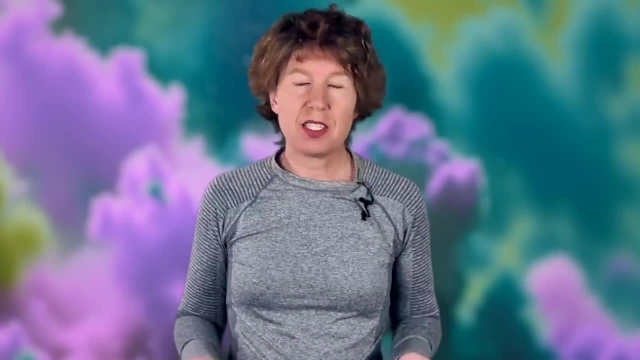 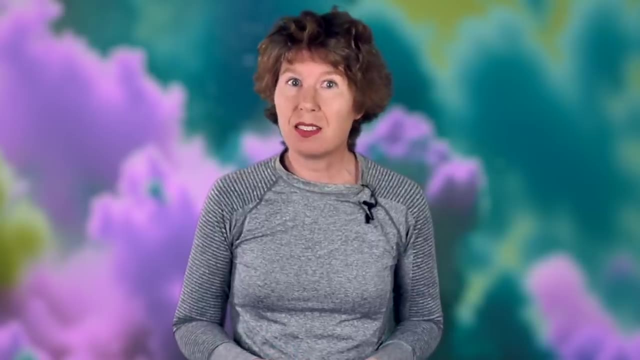 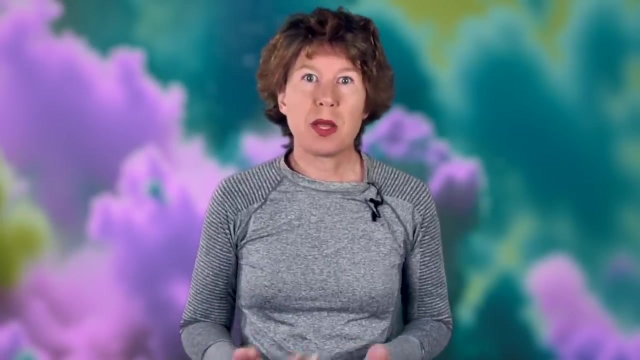 It can only go downhill from here. Big questions like this got me interested in physics. The fascinating thing about them is that you don't need all that much maths to understand them. It's differential equations and probabilities and that's basically it. If you want to know more about the maths behind what I talked about today, I recommend you. 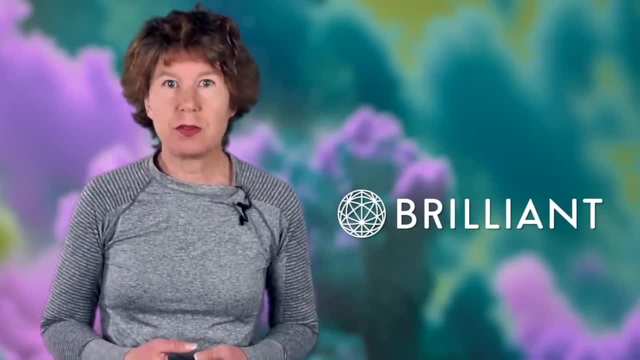 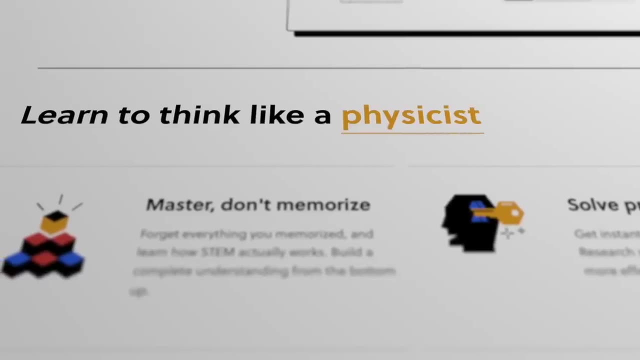 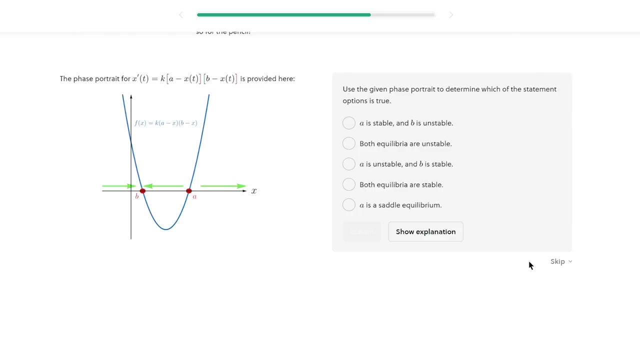 try Brilliantorg, who have been sponsoring this video. Brilliant offers courses on a large variety of topics in science and mathematics. They have excellent courses on differential equations, as well as on the fundamentals of statistics and knowledge and uncertainty. Like all their courses, they come with interactive visualizations and follow-up questions. so 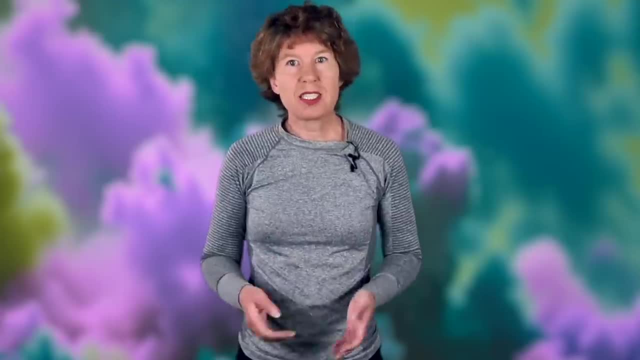 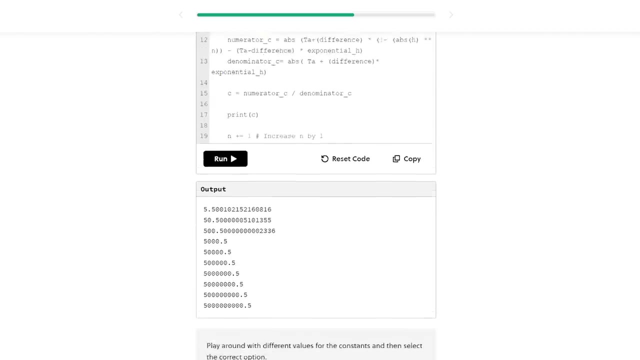 you can check your understanding right away. Brilliant is a fresh and new approach to learning. I wish it had been around when I was a kid. I wish I had been able to do it. I wish I was a student, because I've found it highly effective to understand and also. 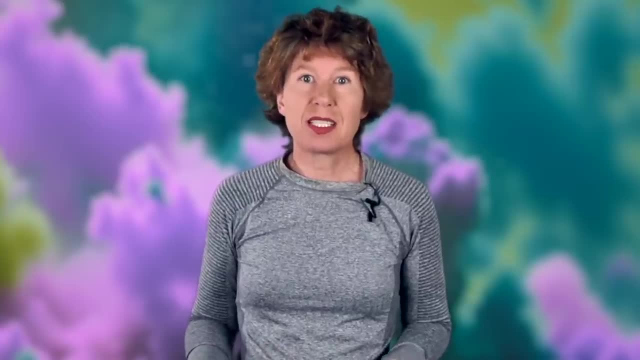 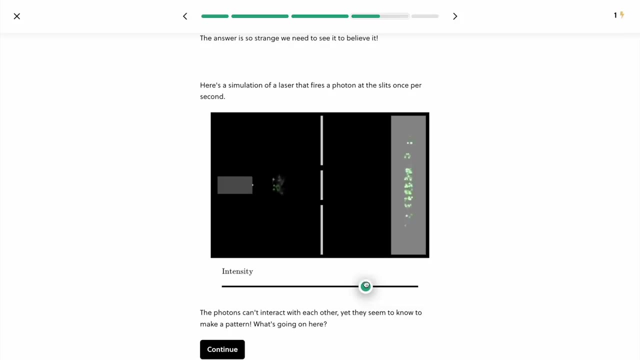 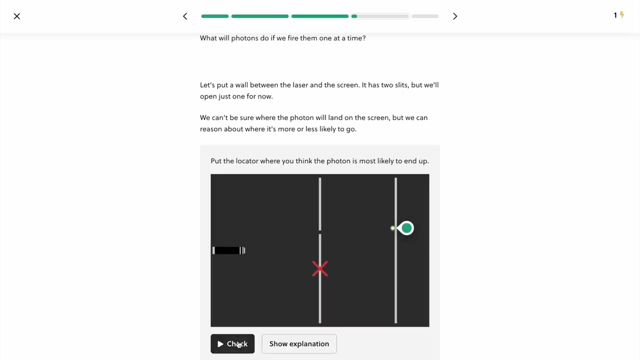 remember material. I even have my own course on Brilliant now. that's an introduction to quantum mechanics. It starts from the very basics and doesn't require you to bring background knowledge. My course covers topics such as interference, superpositions and entanglement. the uncertainty